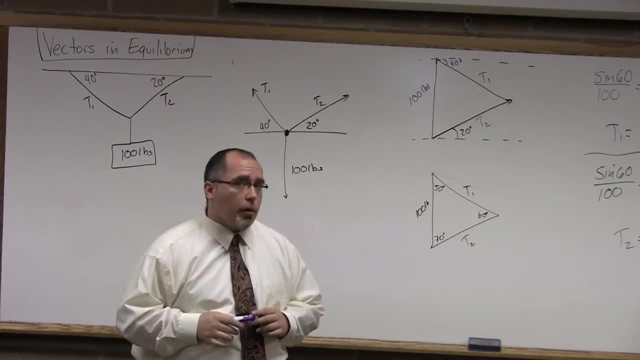 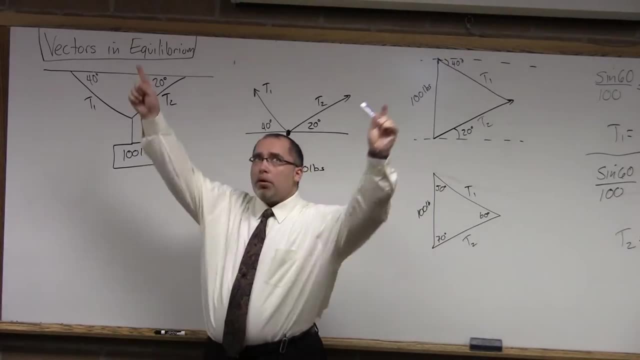 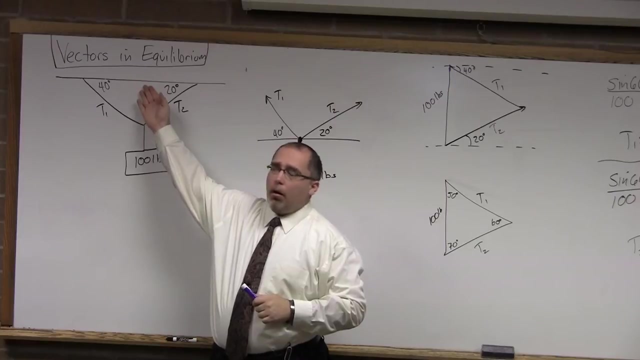 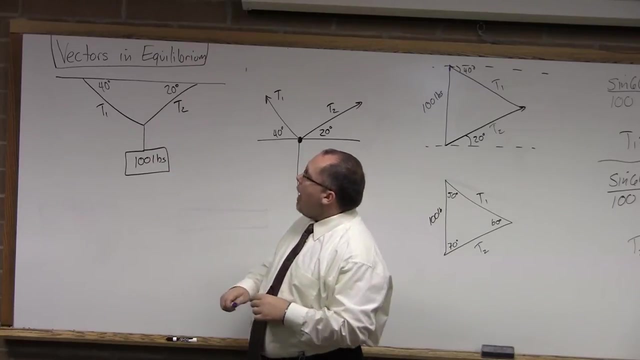 Hello again, In this video we're going to talk about vectors in equilibrium. Now what vectors in equilibrium are, and here's a good diagram to represent it. Say, for instance, you had something you wanted to suspend from the ceiling like a chandelier or something to that effect, But there was something right above it and you couldn't anchor it in there. So you have two different cords coming down suspending this chandelier or whatever it happens to be- And it was a hundred pound chandelier- and this cord created a four degree view. 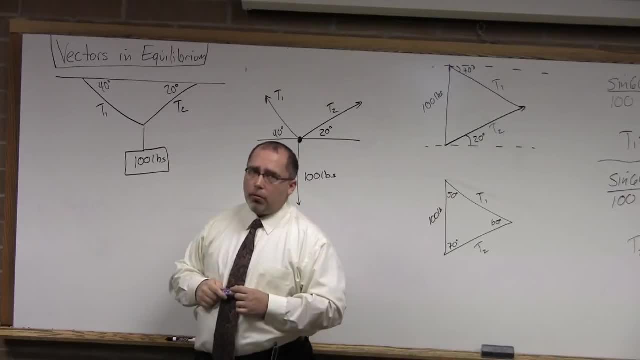 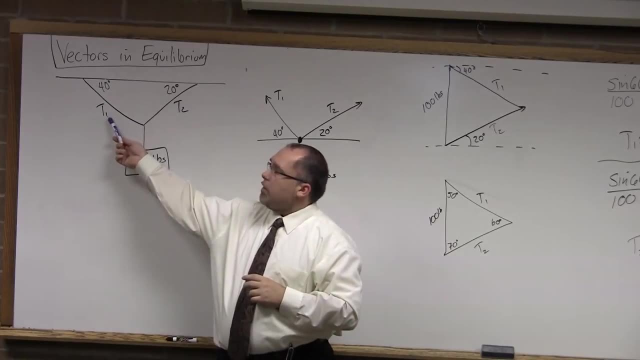 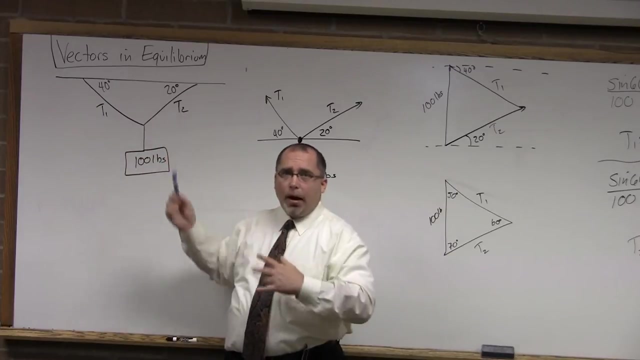 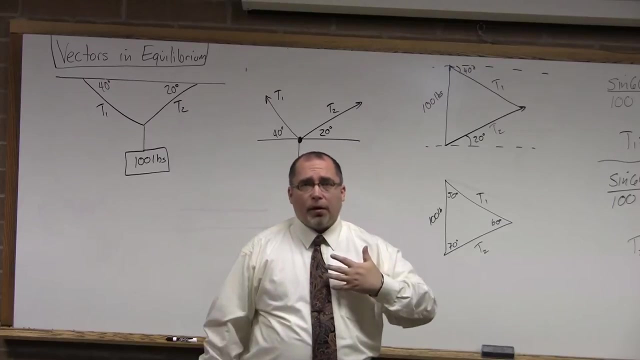 This cord created a 20 degree angle with the ceiling. This cord created a 20 degree angle with the ceiling. Another form of force is tension in a rope or cord or whatever. So we're going to call this cord one. So T1 represents a tension in cord one, T2 represents a tension in cord two. This is our real world diagram. We're going to go from that to a vector diagram, like we discussed before, Where now the length of the vector is representative of the force or the magnitude of the force, In this case the magnitude of the tension. 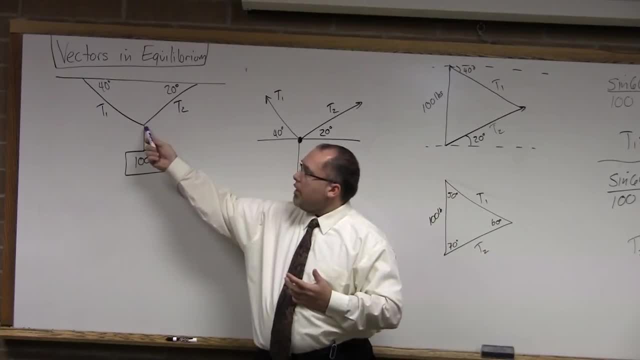 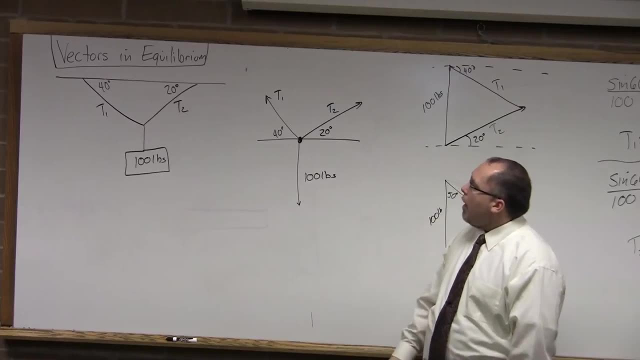 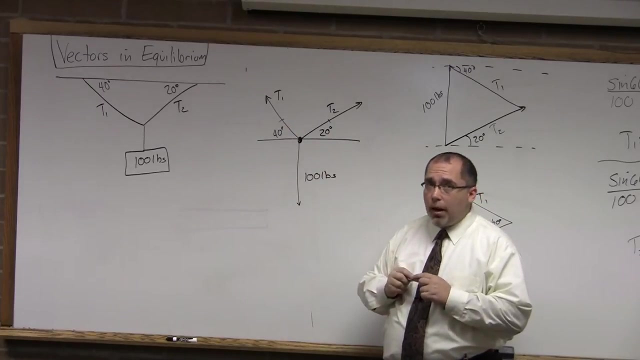 So all three of these cords meet at this one point. That point is here. We then have a hundred pound vector going straight down- That's the weight of the chandelier- And we have T1 going off at a 40 degree angle to the horizontal, T2 off to a 20 degree angle to the horizontal. What we're going to do here is we're actually going to solve for the length of T1 and T2.. Because, remember, the length of the vector, again, is representative of the magnitude, or the numerical value of the vector, Or how many pounds of tension. 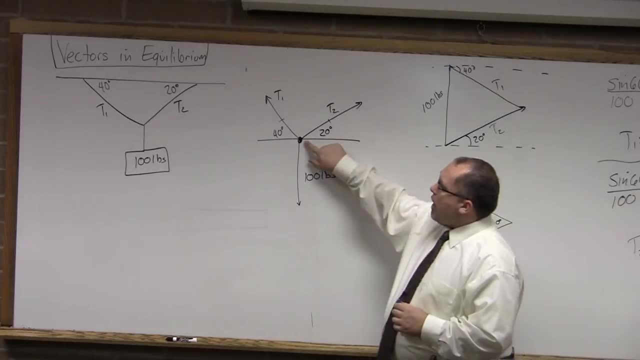 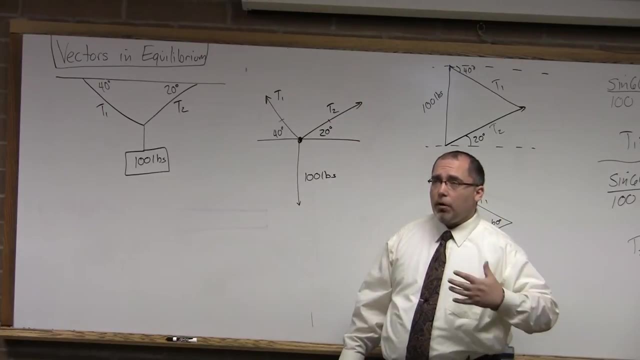 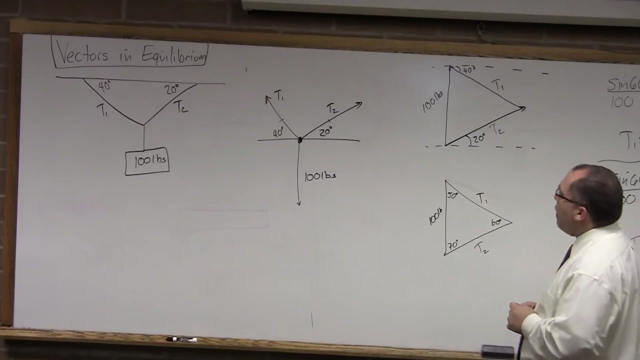 Are in that vector. So what we're going to do is we're going to separate each of these three vectors from this point. We're going to rearrange them to form a triangle, Because the past couple modules- we talked about right and oblique triangles and how to solve for sides and angles, And remember now the lengths of these vectors that will become the size of a triangle are again representative of the magnitude of the force in that tension. So we arrange them. We put the hundred pound vector straight, vertical there, And if it's a vertical vector in all ways, 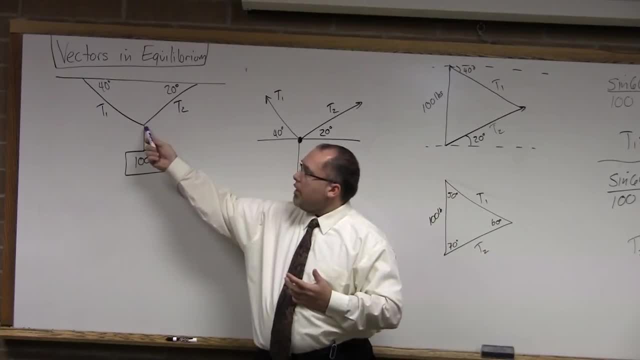 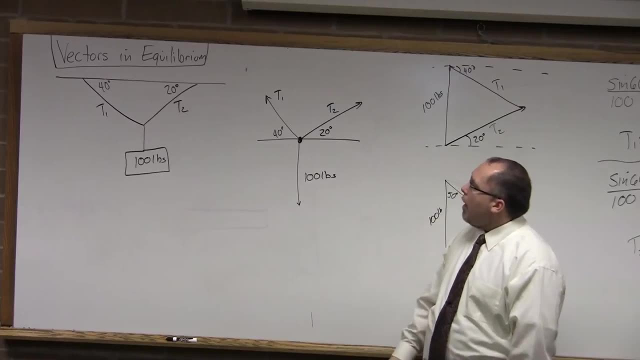 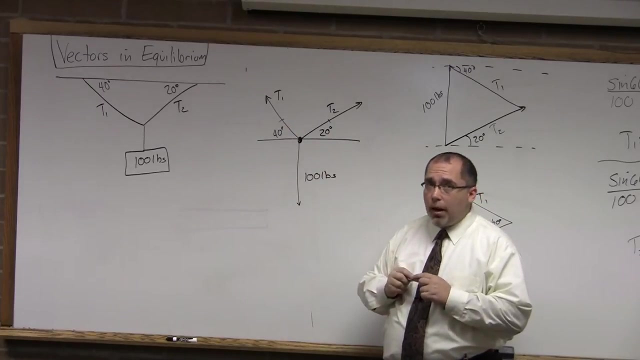 So all three of these cords meet at this one point. That point is here. We then have a hundred pound vector going straight down- That's the weight of the chandelier- And we have T1 going off at a 40 degree angle to the horizontal, T2 off to a 20 degree angle to the horizontal. What we're going to do here is we're actually going to solve for the length of T1 and T2.. Because, remember, the length of the vector, again, is representative of the magnitude, or the numerical value of the vector, Or how many pounds of tension. 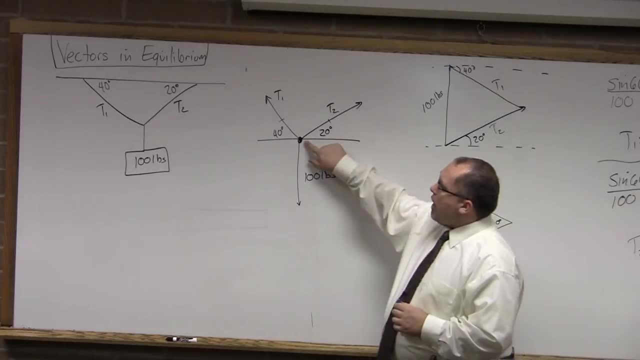 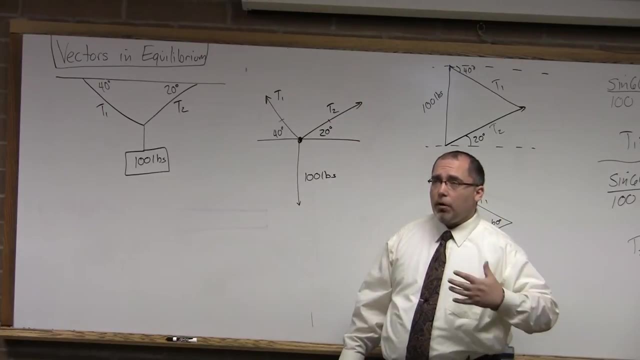 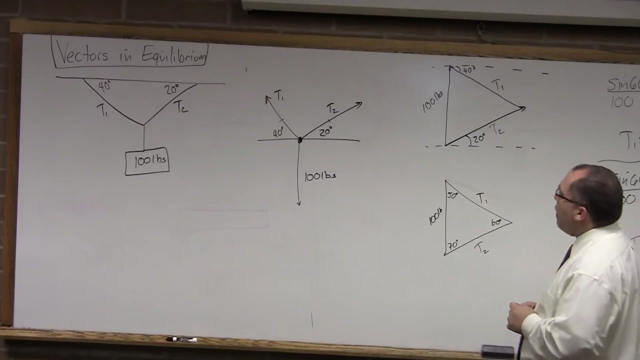 Are in that vector. So what we're going to do is we're going to separate each of these three vectors from this point. We're going to rearrange them to form a triangle, Because the past couple modules- we talked about right and oblique triangles and how to solve for sides and angles, And remember now the lengths of these vectors that will become the size of a triangle are again representative of the magnitude of the force in that tension. So we arrange them. We put the hundred pound vector straight, vertical there, And if it's a vertical vector in all ways, 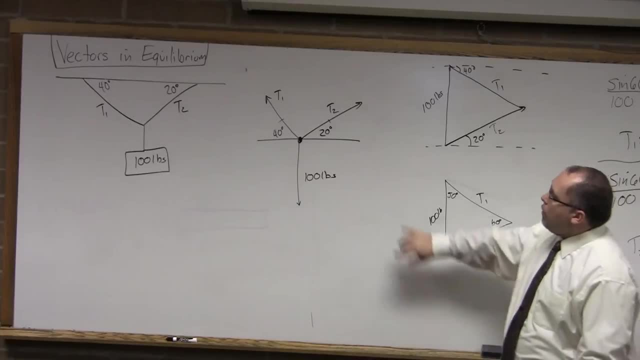 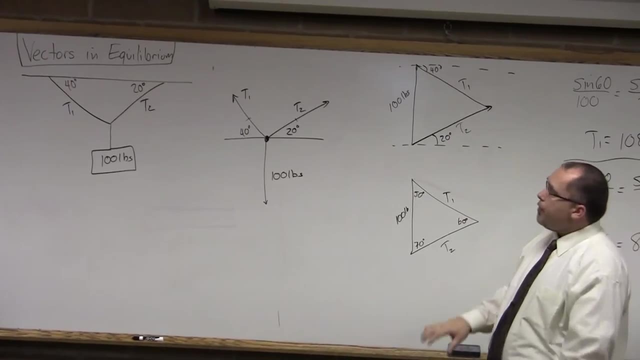 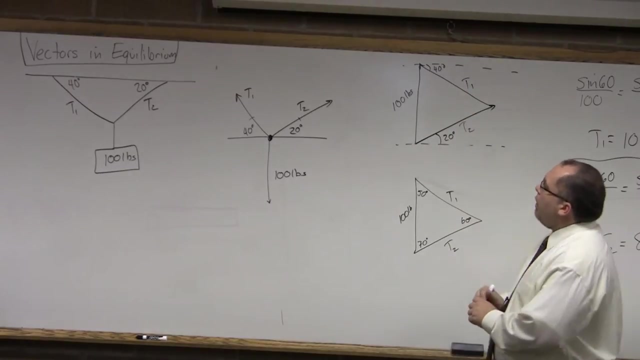 The way vectors are is perpendicular to any horizontal. We're then going to take T2 and we're just going to slide it right here at the same angle. It's like rearranging pieces of a puzzle: T1, we're going to slide and put it right here. So now we form a triangle And again we have one side of the triangle. We're solving for the other two sides The angles. for instance, T2 is at 20 degrees to the horizontal. It is still at a 20 degree angle to the horizontal. 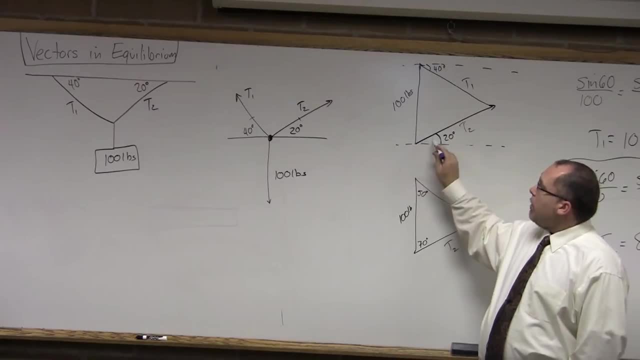 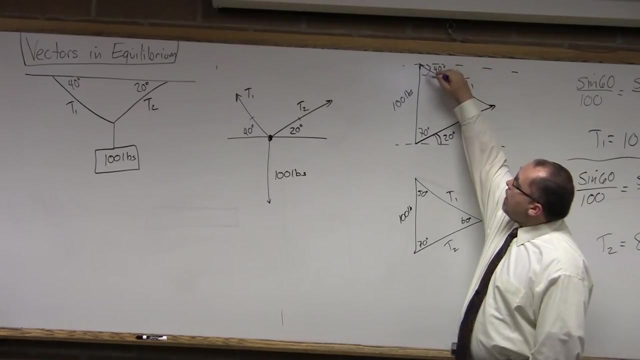 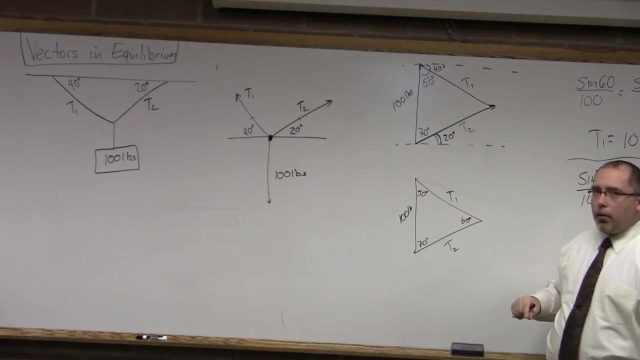 But since this hundred pound vector is perpendicular, If you have 20 degrees outside, there's going to be 90 minus 20 or 70 degrees inside. Likewise, with T1 tacked on here, it's still 40 degrees to the horizontal. So if you take 90 minus 40, that gives you a 50 degree angle to the horizontal. To clean up a bit, I just do the triangle with a hundred pound vector there, A hundred pound side, 50 degrees there. 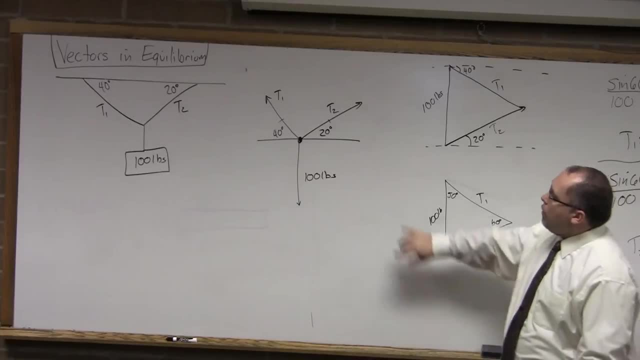 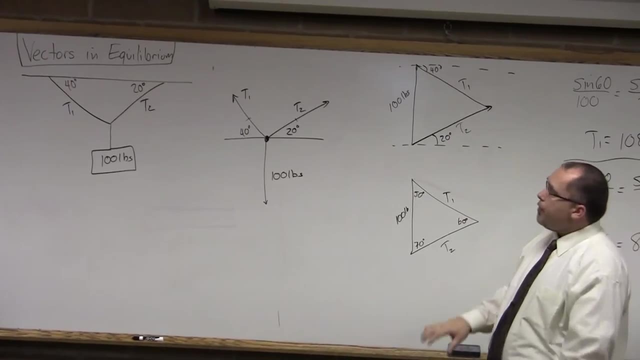 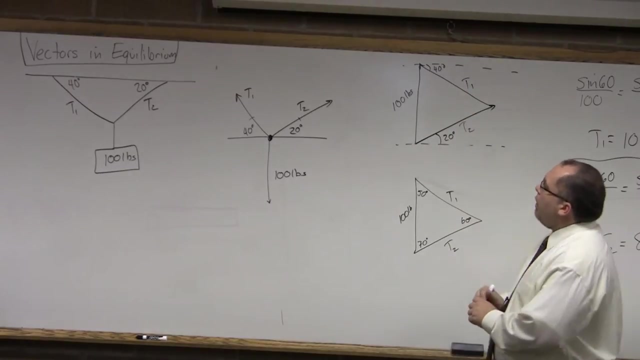 The way vectors are is perpendicular to any horizontal. We're then going to take T2 and we're just going to slide it right here at the same angle. It's like rearranging pieces of a puzzle: T1, we're going to slide and put it right here. So now we form a triangle And again we have one side of the triangle. We're solving for the other two sides The angles. for instance, T2 is at 20 degrees to the horizontal. It is still at a 20 degree angle to the horizontal. 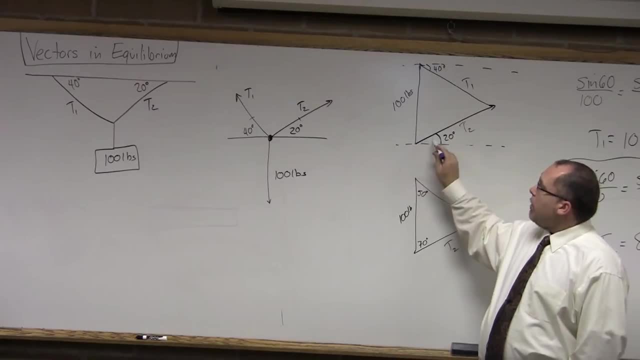 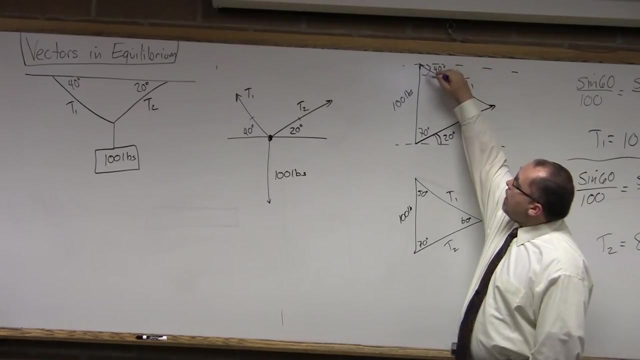 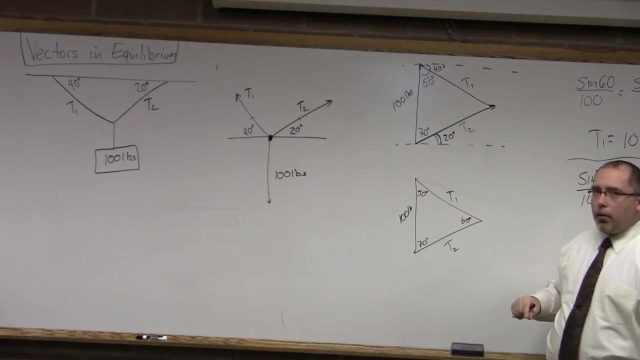 But since this hundred pound vector is perpendicular, If you have 20 degrees outside, there's going to be 90 minus 20 or 70 degrees inside. Likewise, with T1 tacked on here, it's still 40 degrees to the horizontal. So if you take 90 minus 40, that gives you a 50 degree angle to the horizontal. To clean up a bit, I just do the triangle with a hundred pound vector there, A hundred pound side, 50 degrees there. 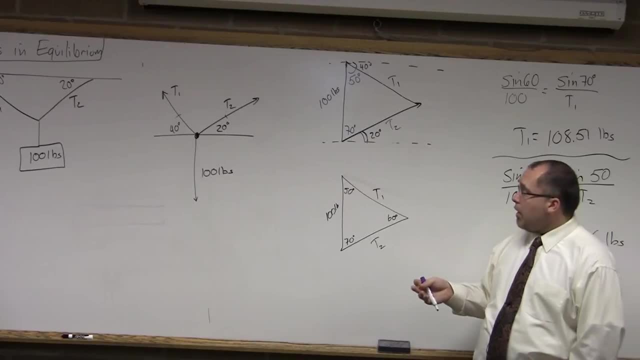 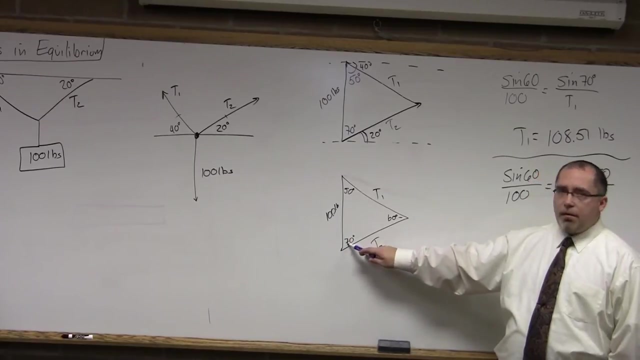 70 degrees there, Remember, all three angles of any triangle always add up to 180. So take 180 minus the sum of these two, which is 120. You have 60 degrees here. You now have a matched pair. Matched pair. If you think back to oblique triangles automatically think of law of sines. So we're going to use law of sines to solve for both T1 and T2 separately. So we have the sine of 60 over 100 equals the sine of 70 degrees over T1. Which is what I have right here. So we have our sine of 60 over 100. 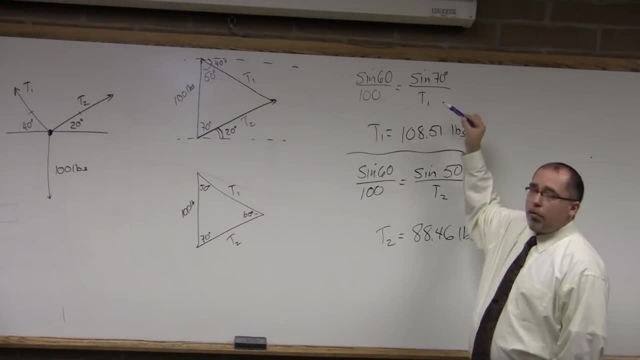 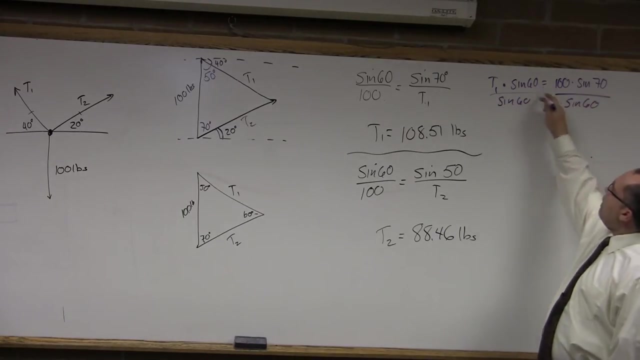 So we have our sine of 60 over 100 equals the sine of 70 over T1. Remember to solve in law of sines you have to cross, multiply. So T1 times the sine of 60 is going to equal 100 times the sine of 70. To get T1 by itself you have to divide both sides by the sine of 60. Those cancel out and T1 would simply be equal to 108.51 pounds. 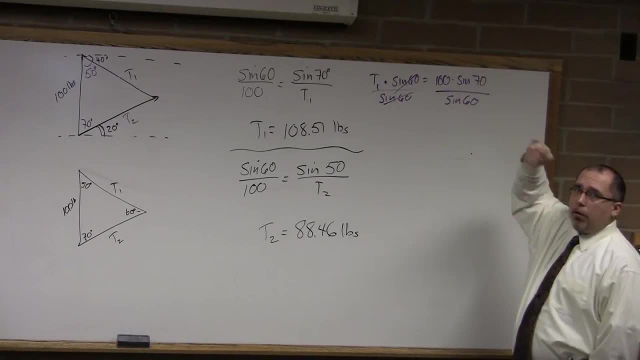 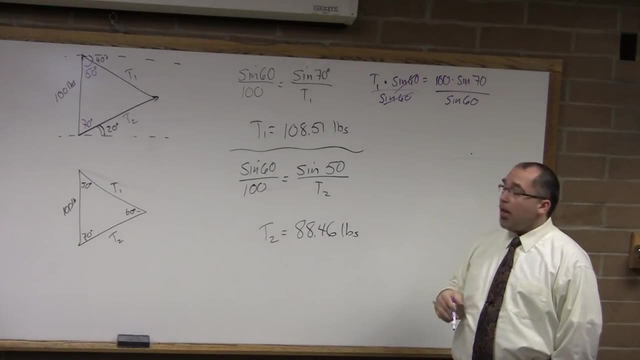 So basically 100 times the sine of 70. Don't forget to close the parentheses after the 70.. Divided by the sine of 60. That gives you 108.51.. So that's how much tension is in chord 1.. 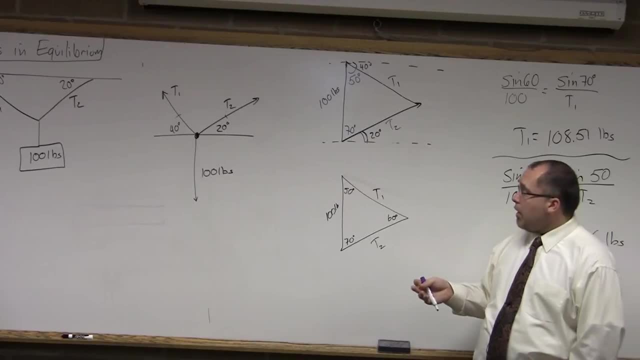 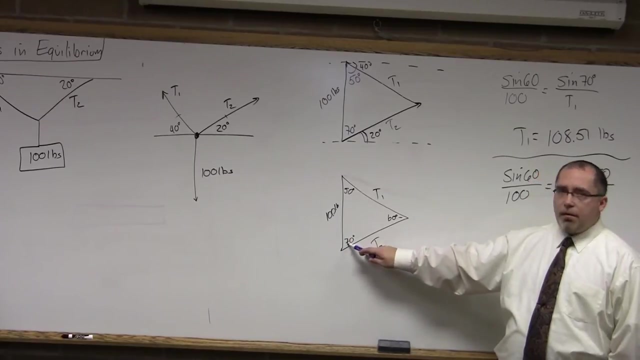 70 degrees there, Remember, all three angles of any triangle always add up to 180. So take 180 minus the sum of these two, which is 120. You have 60 degrees here. You now have a matched pair. Matched pair. If you think back to oblique triangles automatically think of law of sines. So we're going to use law of sines to solve for both T1 and T2 separately. So we have the sine of 60 over 100 equals the sine of 70 degrees over T1. Which is what I have right here. So we have our sine of 60 over 100. 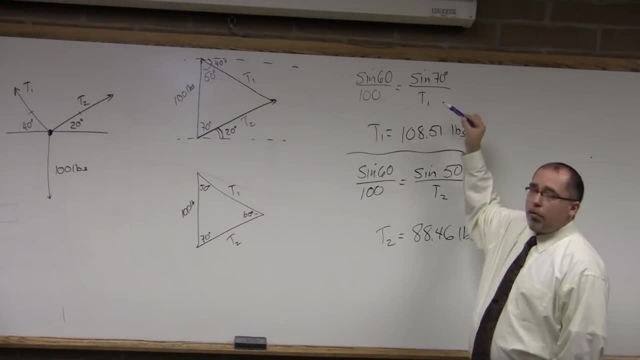 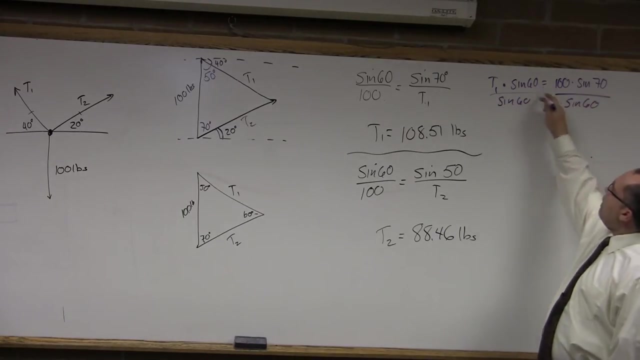 So we have our sine of 60 over 100 equals the sine of 70 over T1. Remember to solve in law of sines you have to cross, multiply. So T1 times the sine of 60 is going to equal 100 times the sine of 70. To get T1 by itself you have to divide both sides by the sine of 60. Those cancel out and T1 would simply be equal to 108.51 pounds. 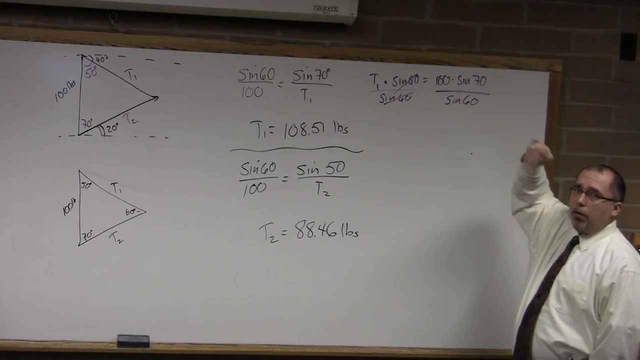 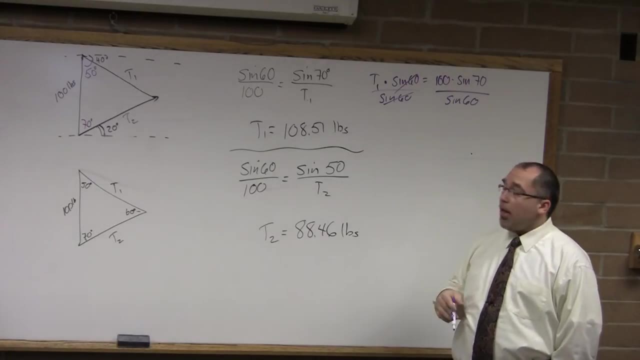 So basically, 100 times the sine of 70. Don't forget to close the parenthesis after the 70.. Divided by the sine of 60. That gives you 108.51.. So that's how much tension is in chord 1.. 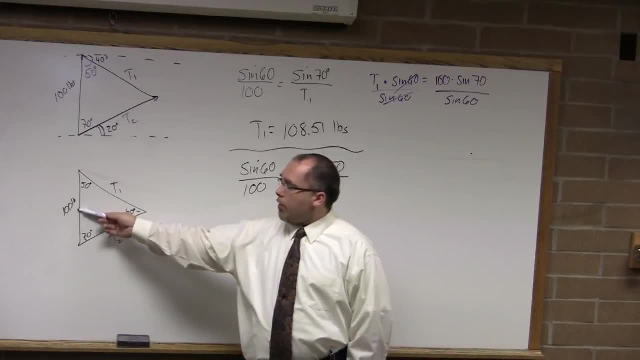 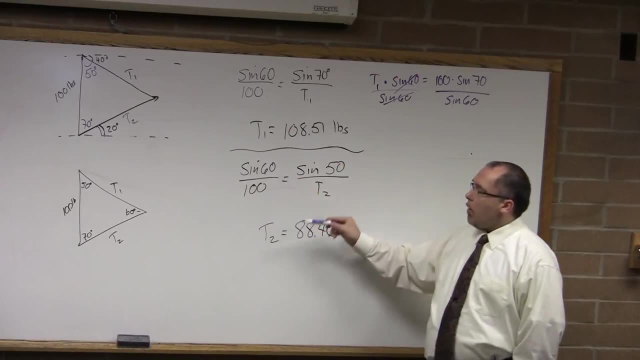 To get T2.. So we take our sine of 60 over 100. But now that equals the sine of 50 degrees over T2.. So we're writing it out: Sine of 60 over 100 equals the sine of 50 over T2.. 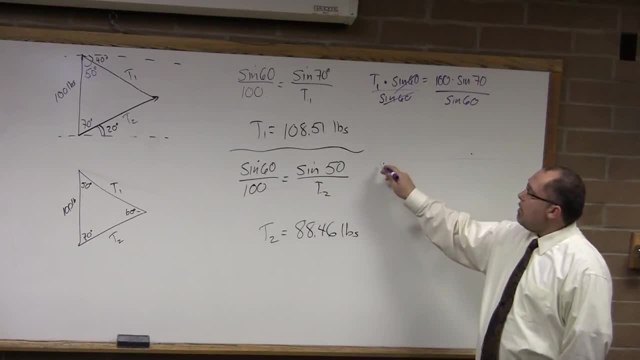 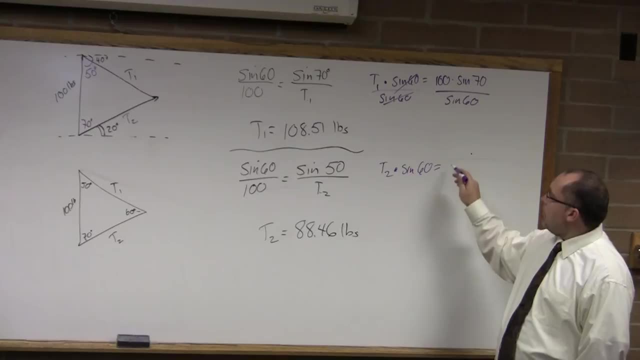 We cross, multiply T2 times the sine of 60.. T2 times the sine of 60.. T2 times the sine of 60.. 60 will then equal 100 times the sine of 50.. To get T2 by itself, divide both sides by: 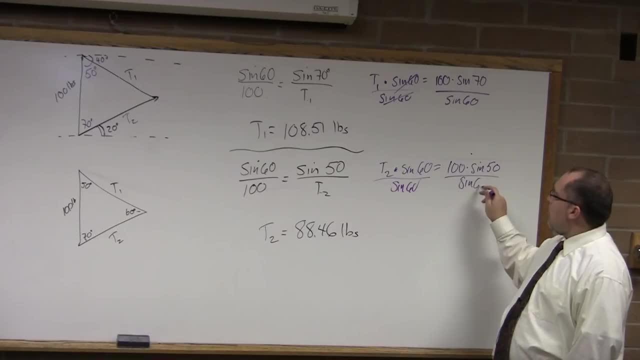 the sine of 60. And if you type that in 100 times the sine of 50, all divided by the sine of 60, you'll get 88.46 pounds. Now you may be thinking: well, this is only a 100-pound. 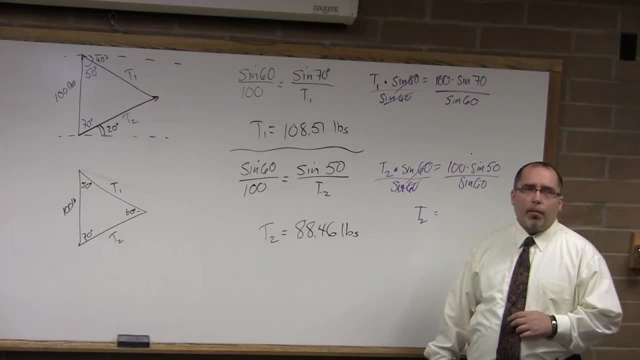 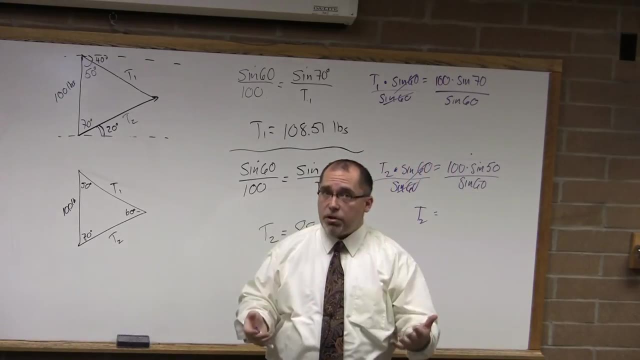 chandelier. Take the sum of these two, you get almost 200 pounds. The thing is, if you had one chord suspending that chandelier, it would only have 100 pounds of tension in it. However, what makes more tension in the chords are the angles that they are to the